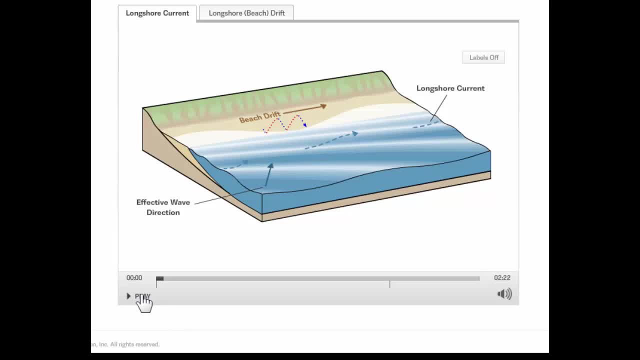 along the beach And this animation illustrates this. You can see here the waves approaching the beach in an angle and as they hit the beach at an angle, they sweep up the beach at an angle and then wash back down up the beach at an angle and wash back down. 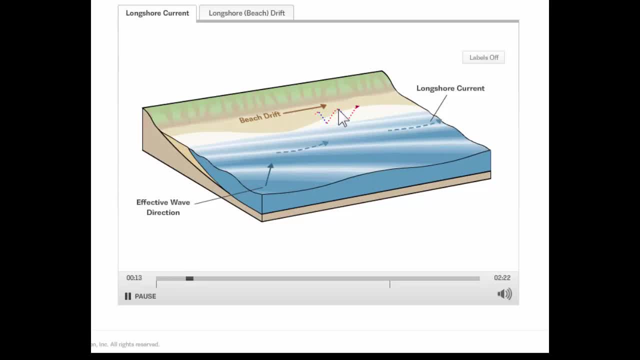 and the result is that the sand moves in a series of zigzaggy arcs along the beach in the direction the beach is at that the waves are going. This is called longshore drift or longshore transport, and the movement of sand occurs not just on the beach itself, but also in this. 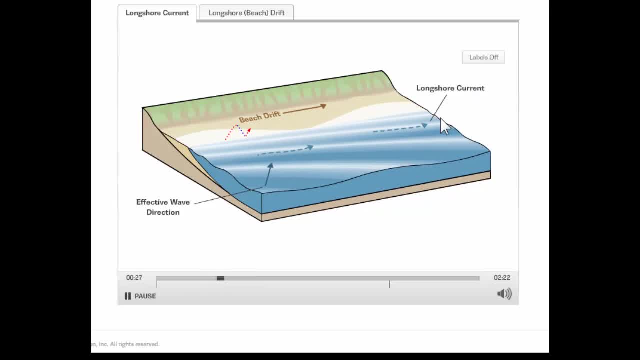 area called the surf zone, before the waves even come to the beach, because the movement of the waves creates a current that's called a longshore current. Now, if you were to go look at the movement of sand by longshore drift along both coasts of the United States, what you would find is the net movement of sand. 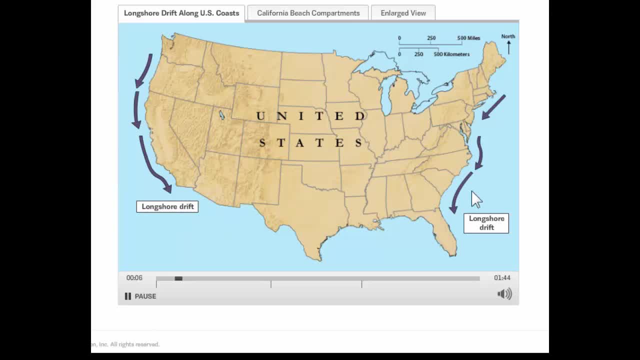 is to the south, both along the west coast and the east coast, And the reason for that is that most of our big waves come from the North Pacific for the west coast, or from the North Atlantic if you're on the east coast. So those waves come from north and they hit the beach from north to south and push. 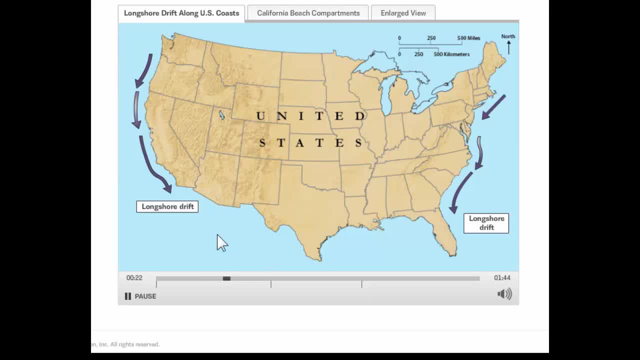 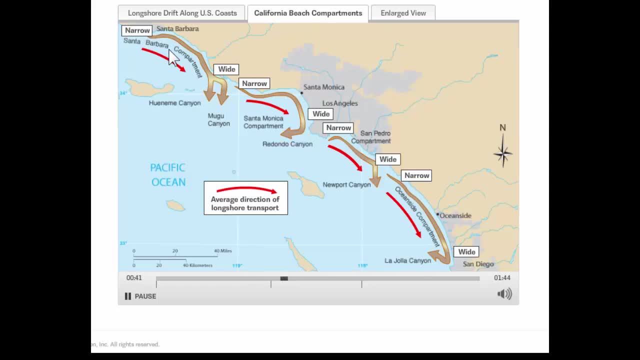 the sand from north to south. Now we're going to go zoom in on Southern California here and look at the movement of sand along our coast. The sand moves south along our coast by longshore drift or southeast because the orientation of the coastline. But what happens is that the movement of sand along our coast 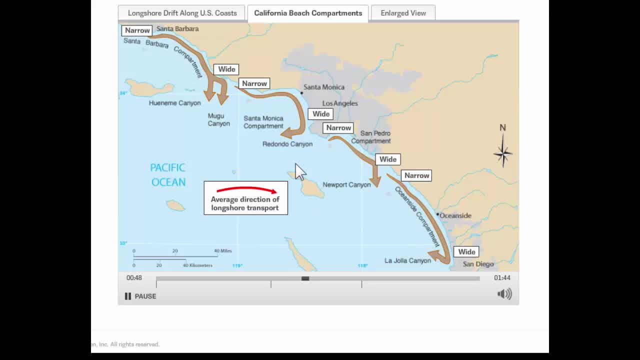 is to the south. So what happens is the sand doesn't just travel south along the coast forever, It ends up leaving the beach, where it drains off down these areas that we call submarine canyons, And you can see them labeled here: Redondo. 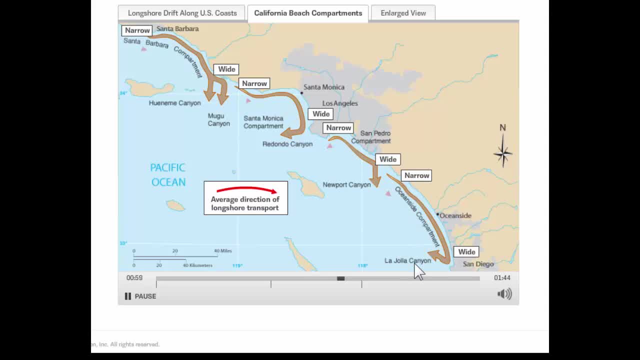 Canyon, Newport Canyon, and then notice La Jolla Canyon down at the bottom of the image there. That's the canyon that is taking all the sand in what's called the Oceanside Beach Compartment. Now, a beach compartment is an area that in 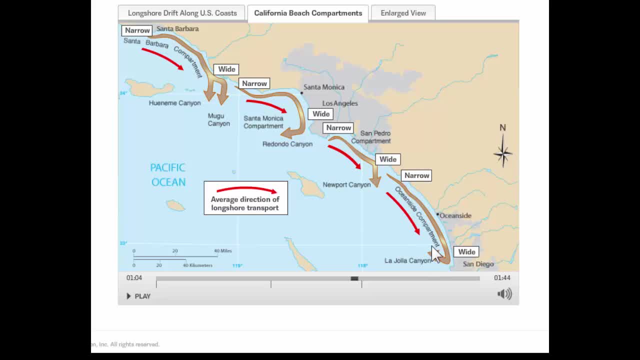 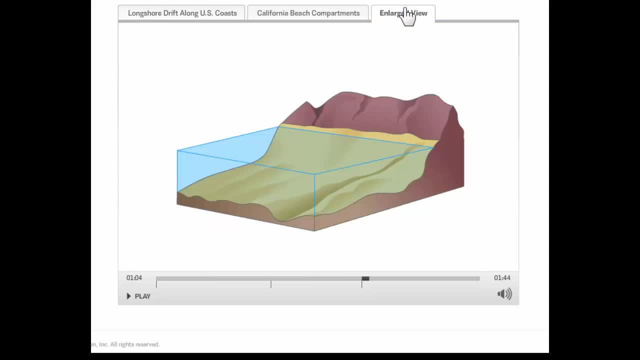 which sand arrives at the beach, moves along the beach and eventually, eventually, reaches down a submarine canyon. And what we're going to go do here is go look more closely at the Oceanside Compartment, at a diagram that will illustrate one of these.